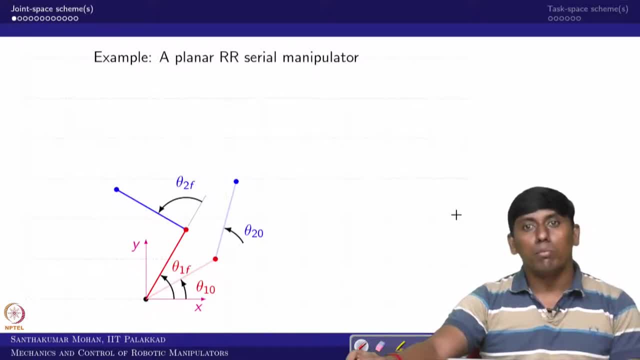 1f and theta 20 supposed to go to theta 2f. that is what we are trying to do. even you have already seen in the lecture. So this can be done In synchronous or probably in series. So we will try to see both in. you can say this. 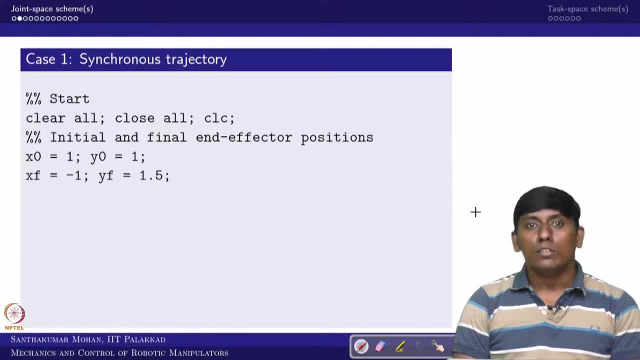 particular lecture. So first one is actually like synchronous, So where we are actually like taking the you call initial position and you can say final position of the end effector. okay, So from there what we can do, we can actually like use the inverse kinematics. 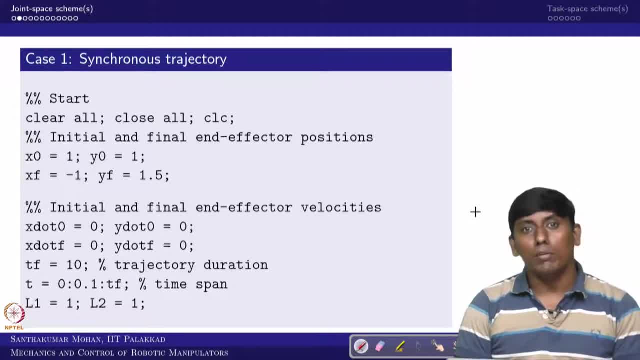 okay, So then we can actually like calculate theta 10 and theta 1f, all those things. So in that connection. So even the initial and final end effector velocity also can be given, because that is what the cubic polynomial all about. If that is the case, we can use the Jacobian in the 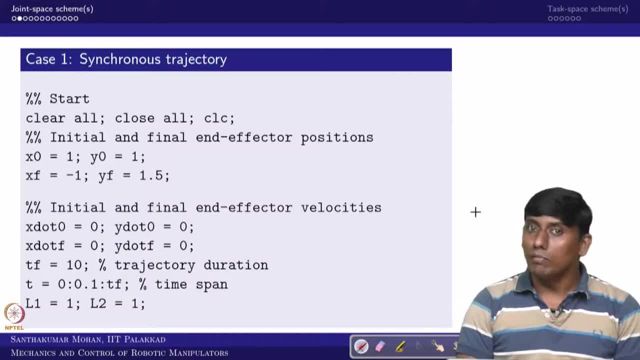 sense the differential kinematics we can use where the inverse differential kinematics we can choose and then try to do it. So, since it is a 2R serial manipulator, the system parameter or the geometric parameter or the physical parameter we need to use, which is we call 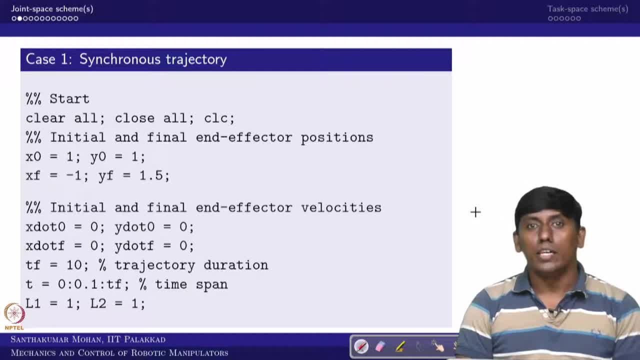 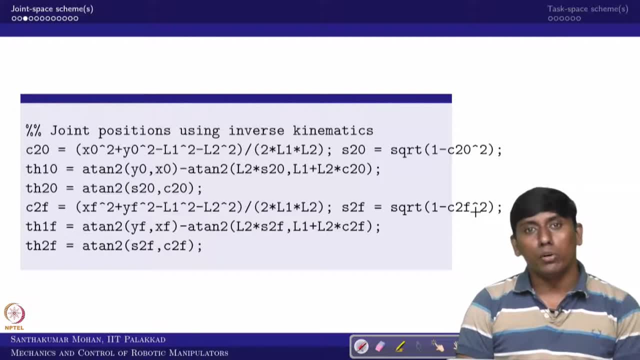 L1 and L2 in this case. So that also we have considered. So now the first case: we are trying to find the inverse kinematics. So we know already inverse kinematics based on the- you can see the closed form equation. So we have used that equation which we derived. 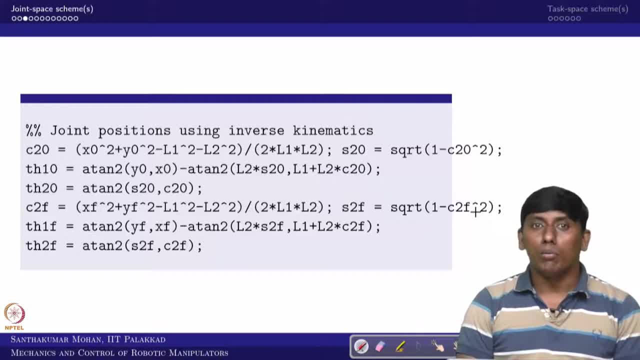 in the regular lecture. So from there we can find theta 10 and theta 20.. So even I would have written as a, you can say, sub function. However, if I write straight away sub function in the math lab, some of you may not be familiar. So that is why I have written explicitly. 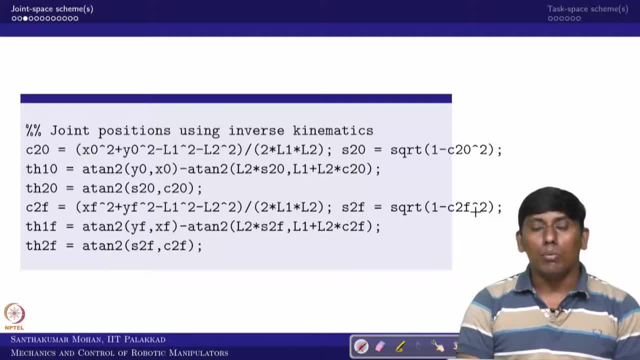 here theta 10, theta 20.. Okay, 2, not then theta 1f and theta 2f. So now what we know? So we know initial and final position of both joints. So now we need to find out the initial and final velocity of each joints. 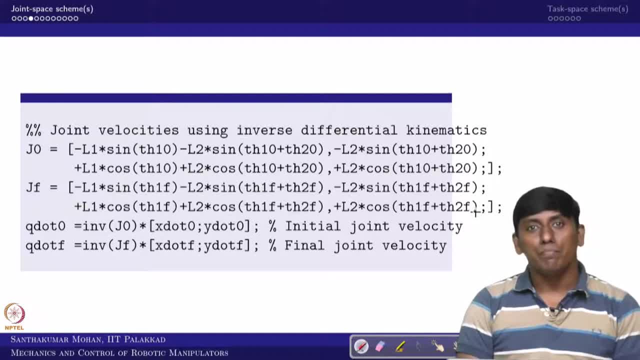 So for that we are taking the Jacobian which we derived in the regular lecture. So now that would be substituted on the initial and final location. So we got J0 and Jf. So based on that- you know already end effector velocities of the initial and final, We can find the 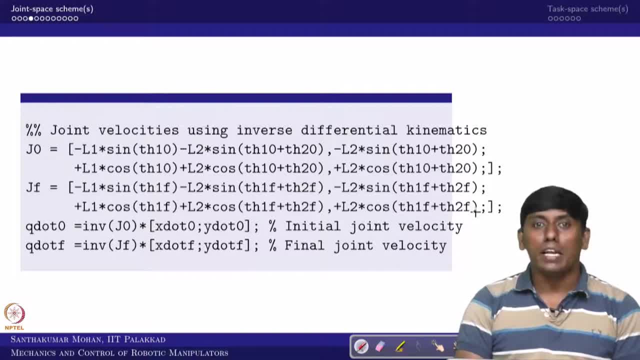 you call theta 1 dot and theta 2 dot for initial and final, which we have written as q dot 0 and q dot f. So once these are all known, then what we can do, We can go back to whatever profile generation you want to use it. So, since it is one of the demonstration I have, 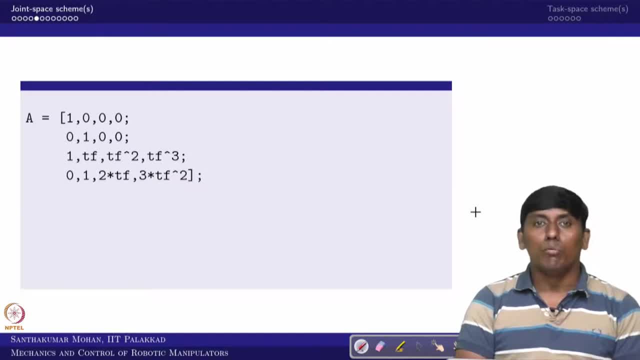 taken as a cubic polynomial. So for that we should know what is we call coefficient matrix A And we should know the, you can say, known input as a vector. So here, the theta 1 initial, theta 1, theta 1 dot initial, theta 1 final and theta 1 dot final need to be known for finding the first segment joint. 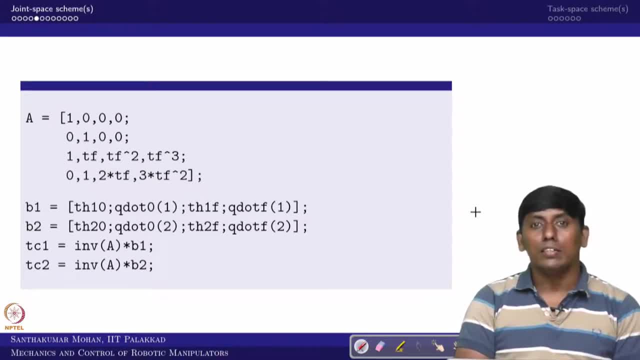 space trajectory. Similarly, second joints- you can say trajectory also- can be generated. So based on that Tc1 and Tc2 for the joint 1 and joint 2 coefficients, which is we call, you can say A0.. So 1 okay to A31, similarly A022 to A32 that we can actually like calculate. So once you, 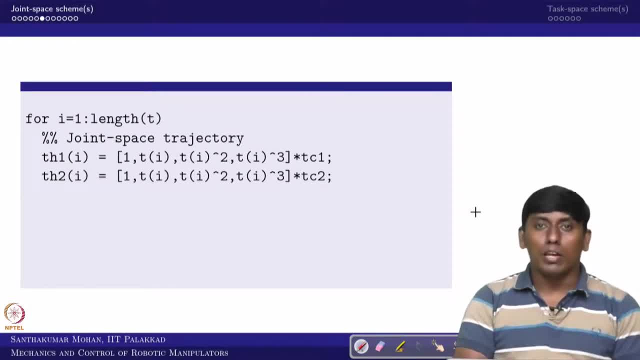 calculate. then we can go to the loop where you are actually like trying to run, based on T0 to Tf profile. So the theta 1 and theta 2 can be generated once you know. since this is a synchronous, So both would be synchronously moving. So in the sense it start from T0 to 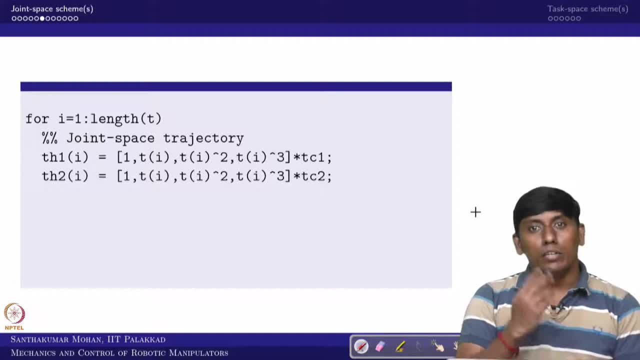 Tf And immediately both joints are rotating. So in that sense we can actually like write theta 1 and theta 2, just to plot as a animated way. So we are trying to find the forward kinematic model so that your X end of vector and Y end of vector can be visualized and 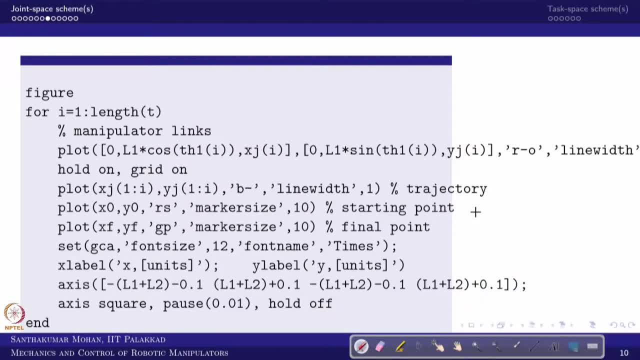 then you can show in a animated way For doing the animation. we have actually like try to take this particular. you can say MATLAB code. So we are actually like trying to plot 0 as the origin, Then X1 and X2.. X1 we can write as L1, cos, theta 1 and X2 is nothing but your final end of vector point. 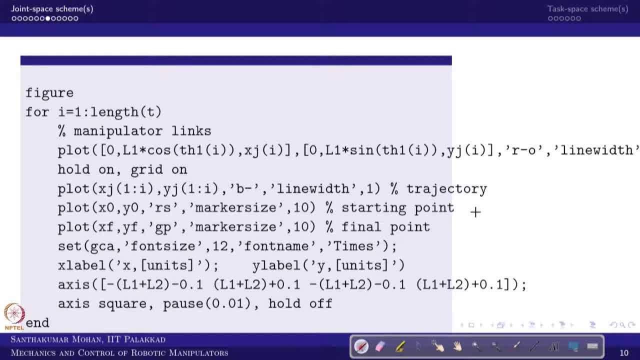 So that is corresponding to the X, Similarly Y. we start from 0 origin, Then L1 sin theta 1 is the Y1 and Y2 would be your end of vector position. So based on that we can draw, and I want to show the continuous profile how it is generated. So I just added that Xj and 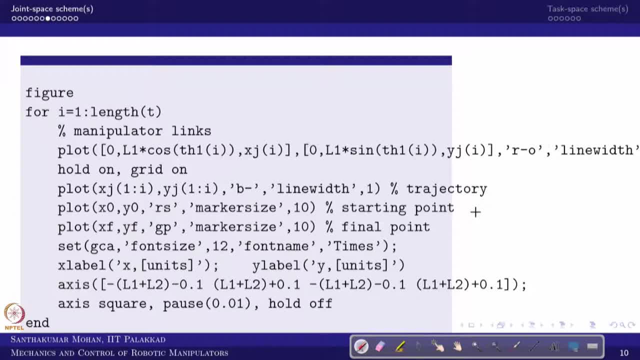 Yj from 1 to I. So when the loop is actually like iterating, it will actually like show the continuous plot and I want to show what is the initial and final point. So I just added to additional plotting where Rs is, the red square will come in the starting point. 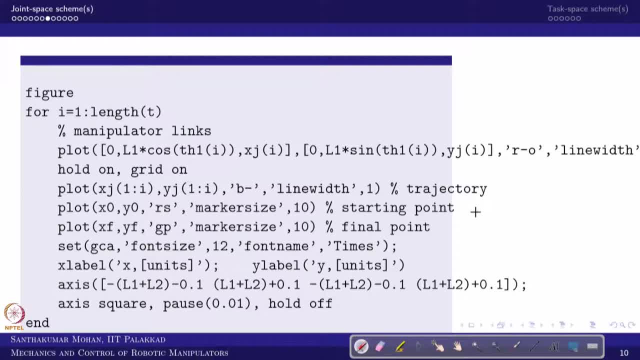 and the GP is nothing. but you can say G, pentagon will, or you can say star will come at the green color at the final point. So, and we have actually like a run everything and just to show the animated, I pass and hold off. So in the sense, every time it would be super impose one image. 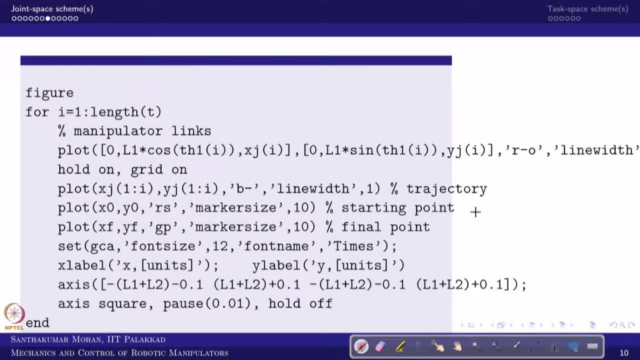 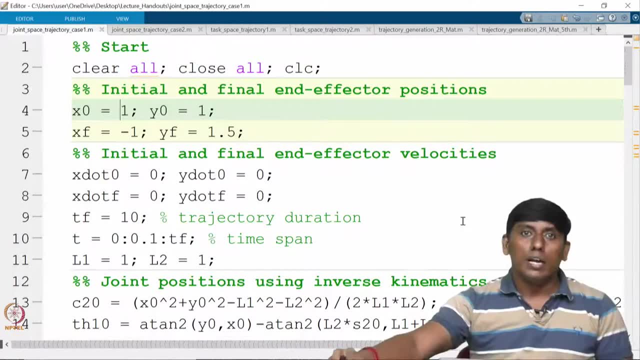 to another image, But hold off command is there, so it is look like as actually a continuous motion. okay, So just to show this, I just go to the MATLAB window and this is the code which we were actually like discussing. So you can see, this is the code. 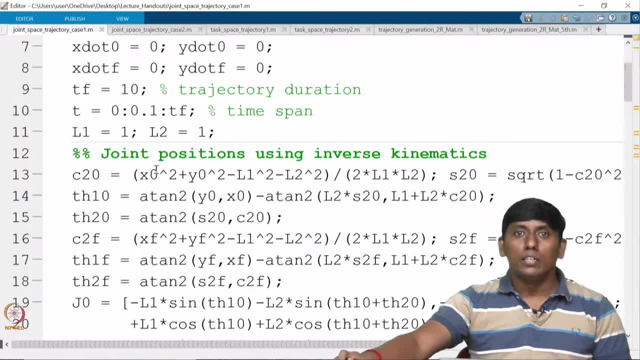 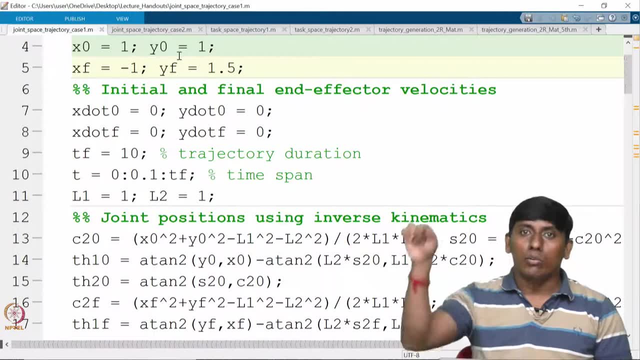 So now, if I run this, so what it start? so the x initial is actually like 1 meter and y initial also like 1 meter. it is actually like somewhere like this and final also like this: So now we have not given theta 1- 0 and theta 1 f directly. 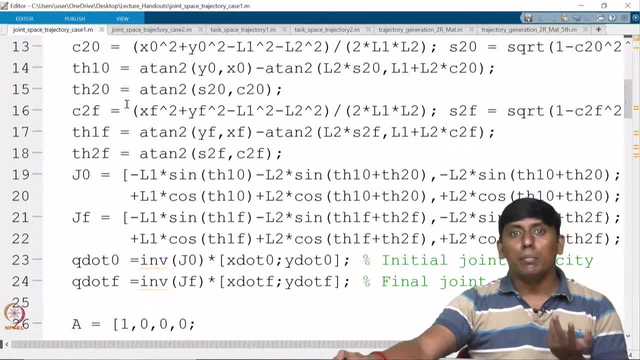 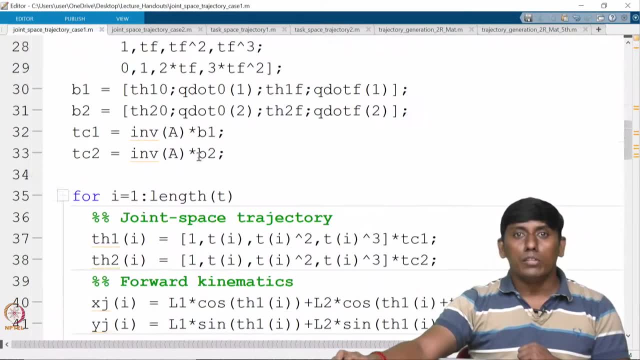 So what we can do, we can do the inverse kinematics. So now the inverse kinematics will have two solution, So we will take one solution, which is the positive solution of S2. okay, So now, based on this, we can actually like run this code. 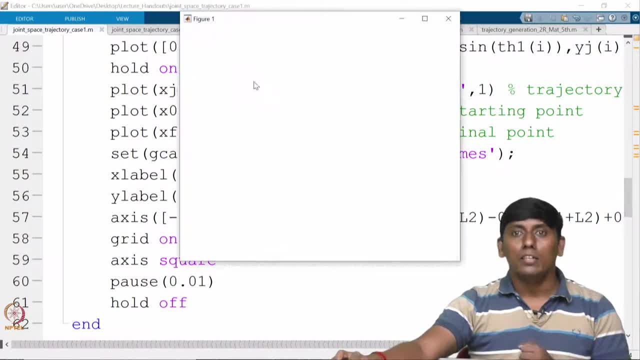 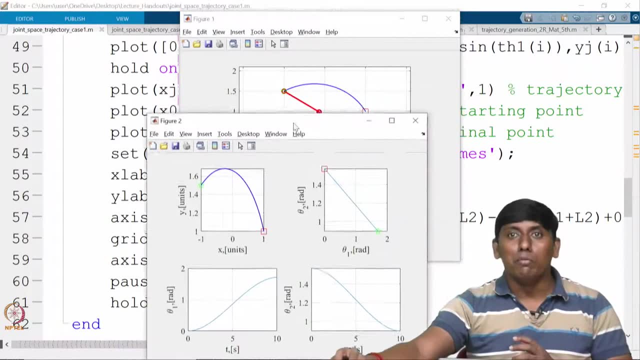 So then you can actually like feel it what I want to actually like explain So you can see like now it is starting from here And it is ending. So you can see like it is more like the robot is actually like moving right, So when I run this, so you can see like the physically the robot is moving, that realization, 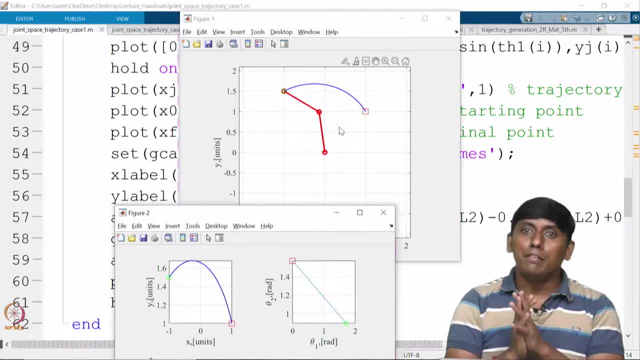 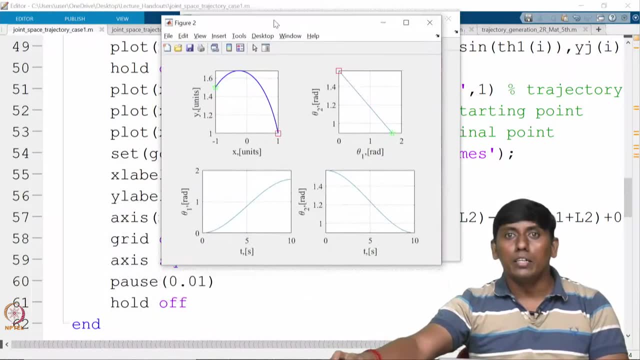 you can feel it in MATLAB animation, So I did not make any video, but still it look like a video, right, because I have made it a superimposed. So the next figure I want to actually like show it. So what is the you can say profile or the trajectory generated in task space and as 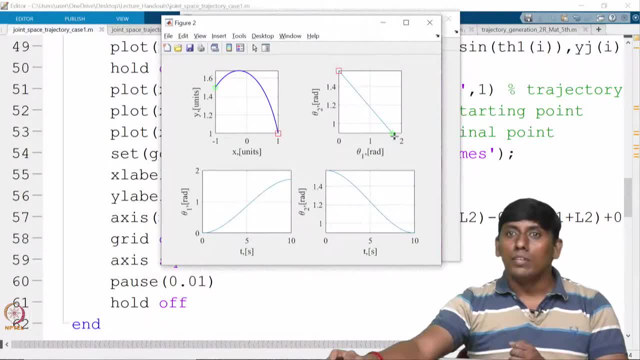 well as the joint space, The joint space theta 1.. Theta 2: you can see it is like a straight line. So that is what we call actually like joint space trajectory. consider as a straight line The profile start from actually like 0 to. you can say this is theta 1, 0 to theta 1 f. 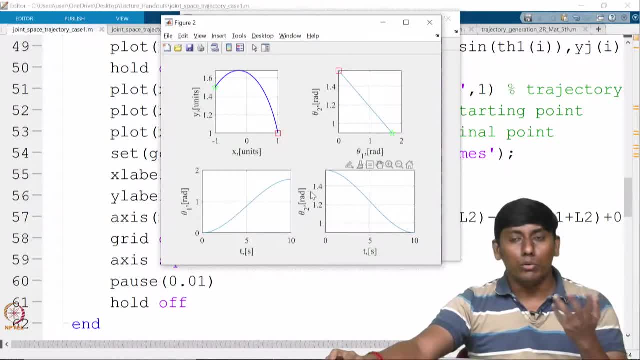 it is a smooth profile And I did not plot the velocity. even you want, you can actually like do the velocity profile. So now, this is the theta 2 f, this is theta 2: 0. So like that we can actually like generate. 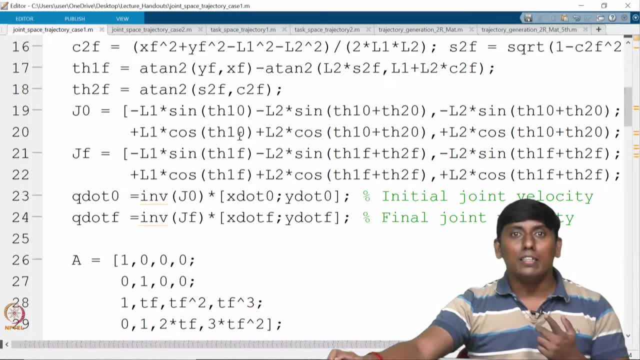 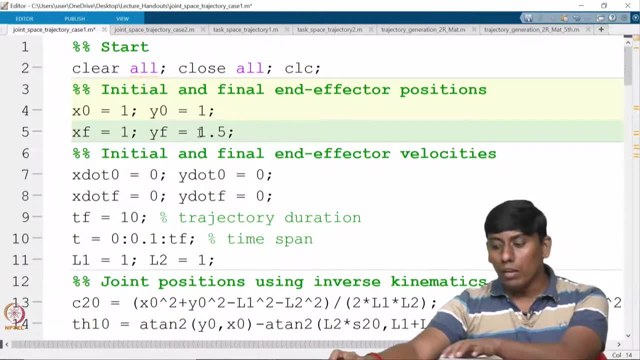 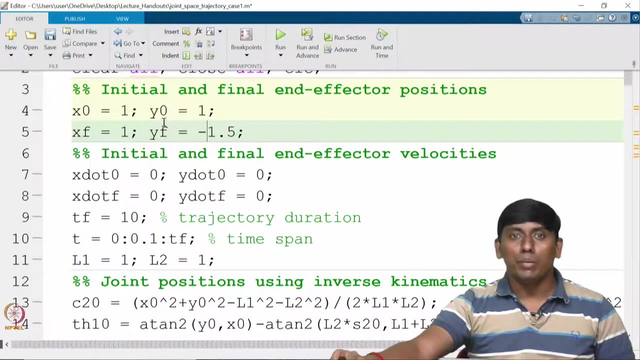 So even you want to actually like realize further. So only condition is this initial input. what we are giving, that should be in the case of what you call in the workspace, So we can actually like see, I have given interchange. So the initial point is same, but the final point is actually like slightly modified. 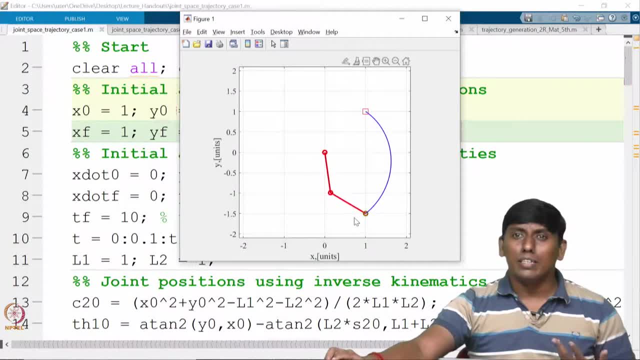 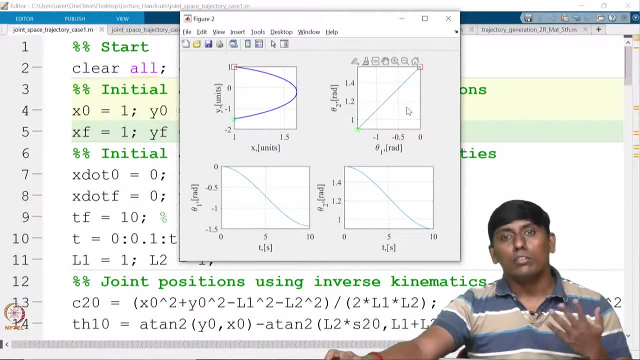 So now you can see that this is the initial point and the final point. You can see it right, it is actually like moving it. So this is what the profile and this is what happening right. So now this is more and more, Actually, like very clear. 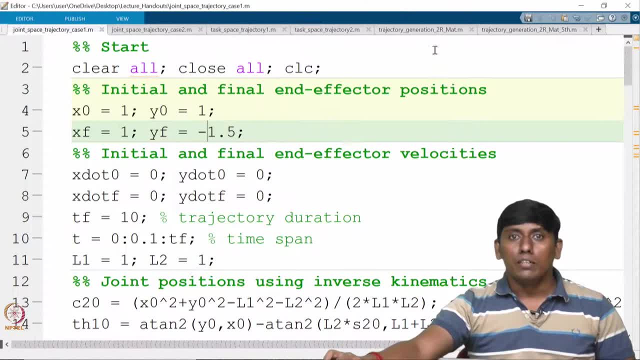 So now we will actually like go back. okay, So go back to the code. So now I am actually like looking at this: okay, So I am just giving it 0 and this is actually like I am putting it, so minus 1.. So now I am actually like trying to give, because your L1 and L2 as 1 and 1.. 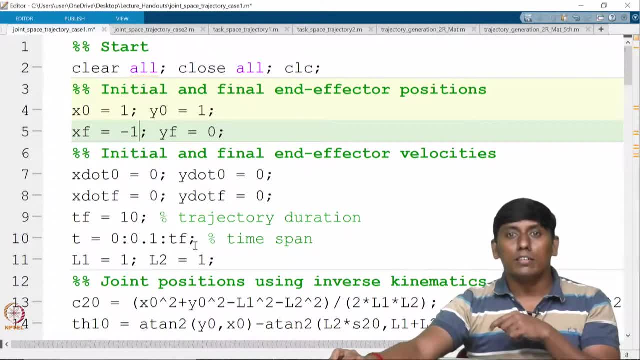 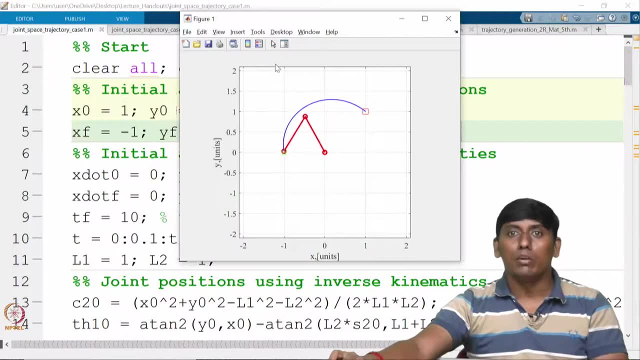 So maximum, it is actually like on the circle of radius of 2 meter, right. So that is what the range, within that you can choose anything. So, anyway, next lecture we would be seeing the workspace generation So you can actually like, feel it right. it is more, more you can say beneficial. 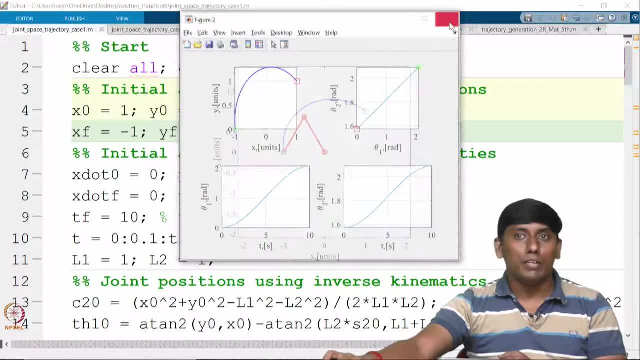 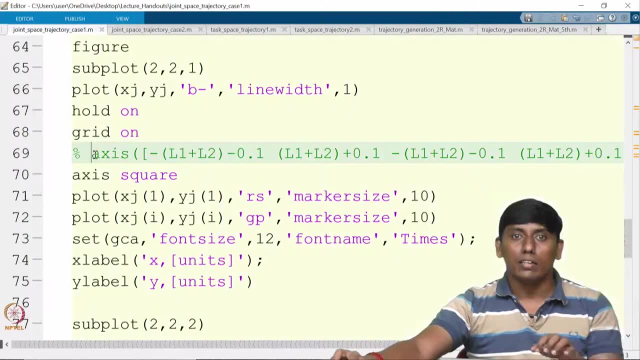 So you want to see this in a proper shape. So even we can actually like make the boundary. So the boundary we can actually like right now I make it this as actually like commented. So now if I actually like make it, it would be giving a real size okay. 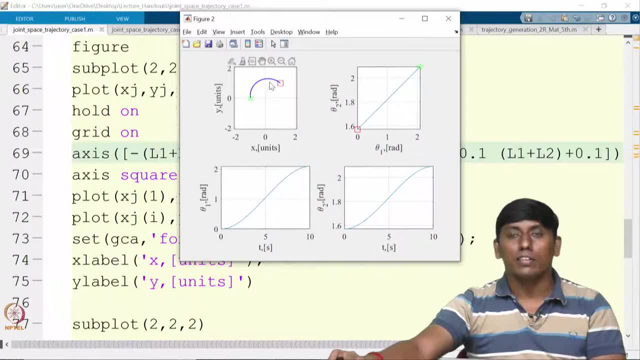 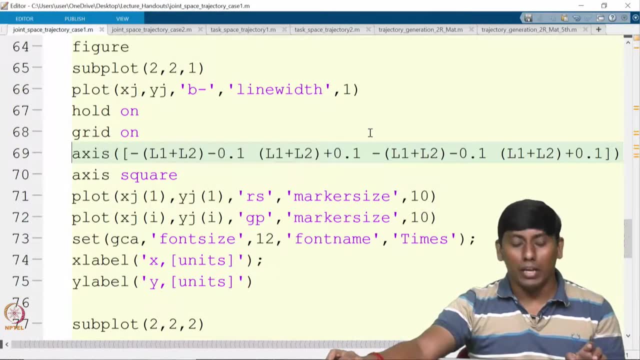 Like how it is happening, the same size it is giving, this is the real size, okay, Okay. So now these all actually like what you call the joint space trajectory, with the case one where the synchronous We will go back to the slide, where the non synchronous we call in series of motion. 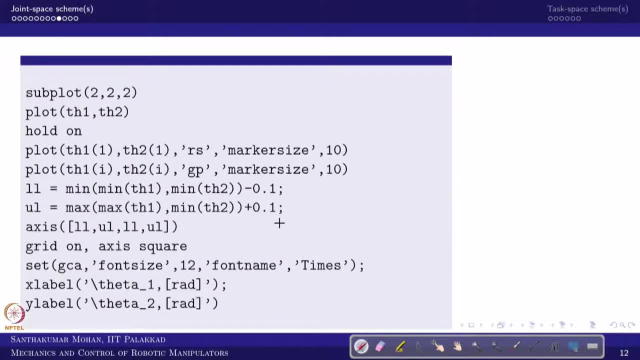 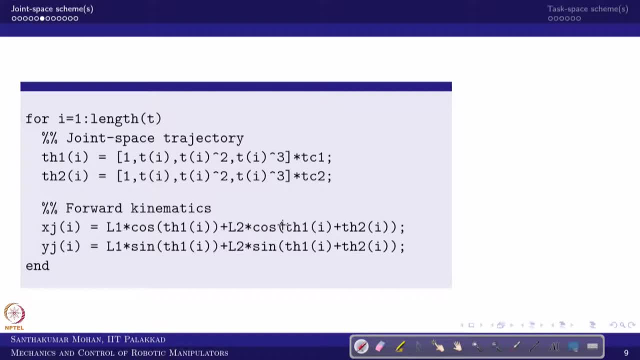 So for that, what we need to actually like, do it. So these all actually like the other plots, okay. So I will just see the non synchronous. So the non synchronous you have to actually like do it slightly a trickier way. So these all the plot which we have already done. 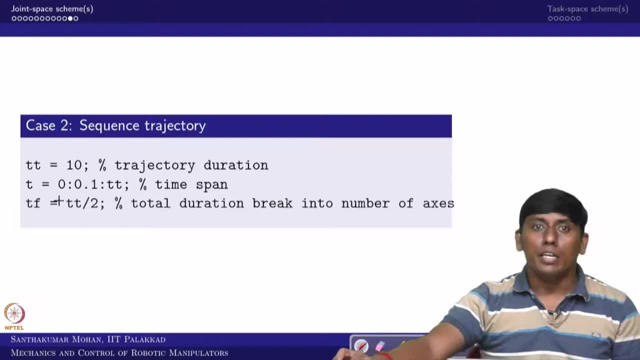 The non synchronous way. it is actually like we call sequence trajectory, So here we call the tt. is that total trajectory duration? But now I need to divide that into tf, into number of segment, because each joint would be rotating independently. for example, now 10 second, I have actually like 2 joints. 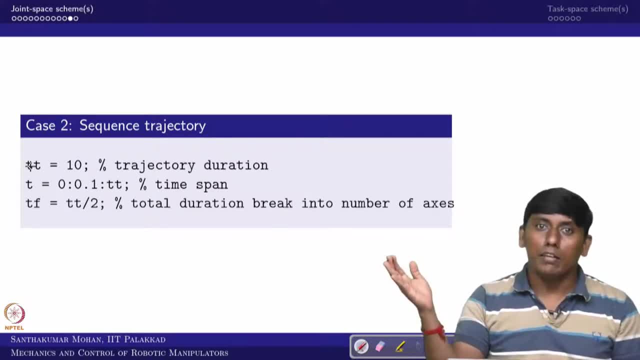 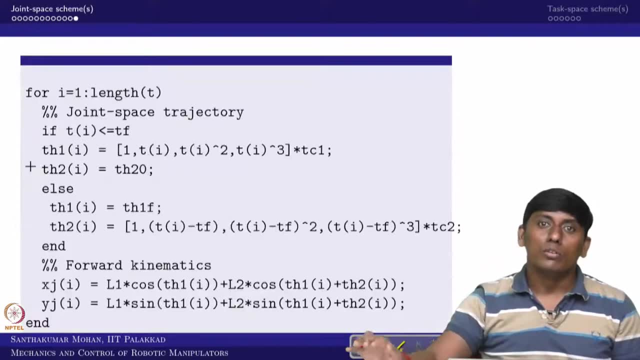 So I actually like break into 5 second each. So first, 5 second first joint will rotate, the next 5 second, the second joint will rotate. So that is what we have seen as a sequence trajectory, So that is what we are trying to see. 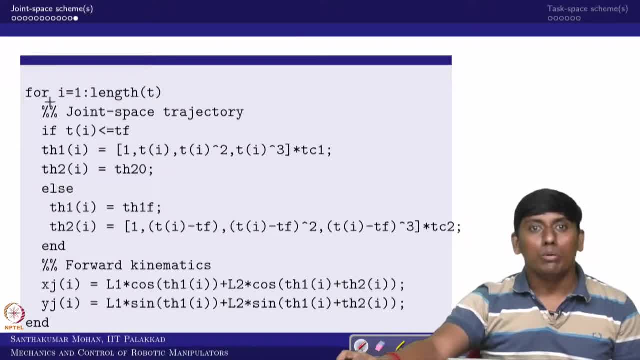 So in the sense the coefficient calculation is same, But what you can see like the t goes 0 to tf. here tf is actually like total duration divided by 2. So that would be generated. So then the correspondingly the theta 2 would be the same initial. it maintain that. 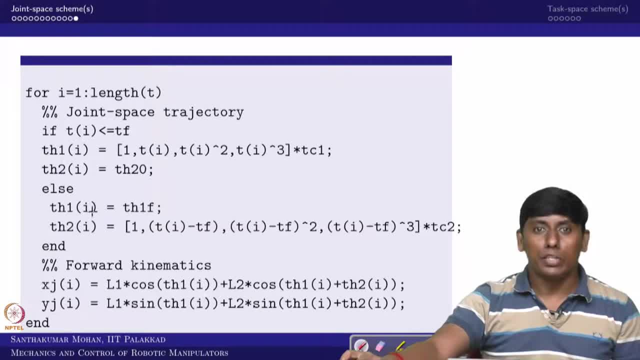 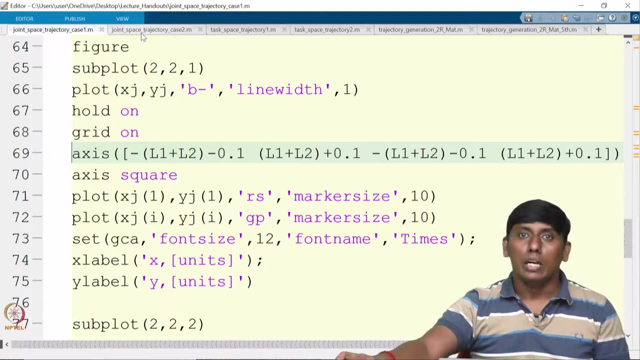 So then you can see the second loop. the final would be maintained for theta 1 and the theta 2 would be move as a cubic polynomial. So now the same way we have done the forward kinematics just to plot, And now we will see the same thing in the MATLAB window, which will give more clear. 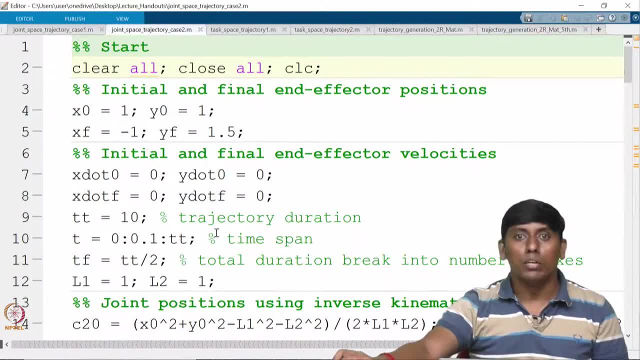 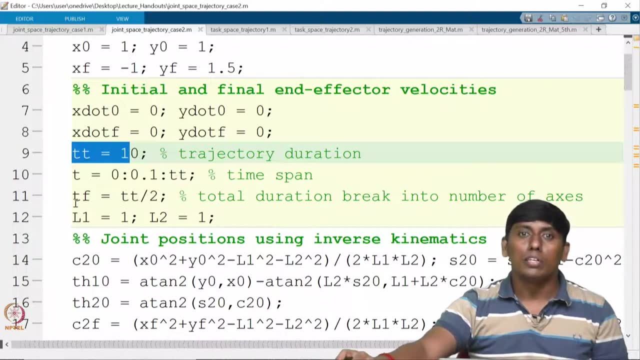 So you can see like these are standard, which we have done in the previous code. Only change is so instead of tf, I have taken tt and the tt and tf. why I have made it? because I make it actually like the tf, always the segment time. the segment time here is actually: 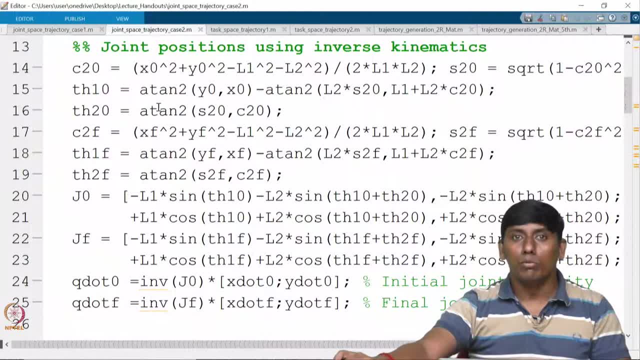 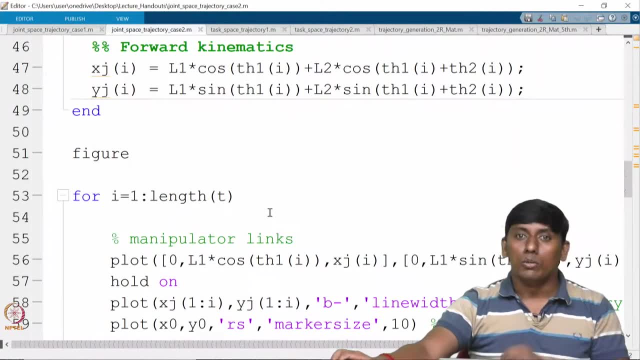 you can say tt divided by 2. So based on that you will get the inverse kinematics and all. So based on that you will get the joint space trajectory in two way. So if I run, you will be very clear to this. So I will just run this. then you will actually like feel it. 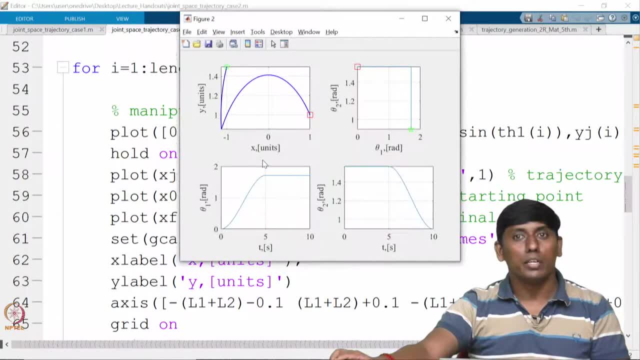 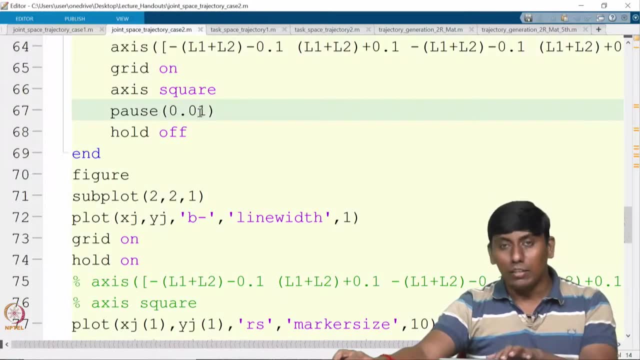 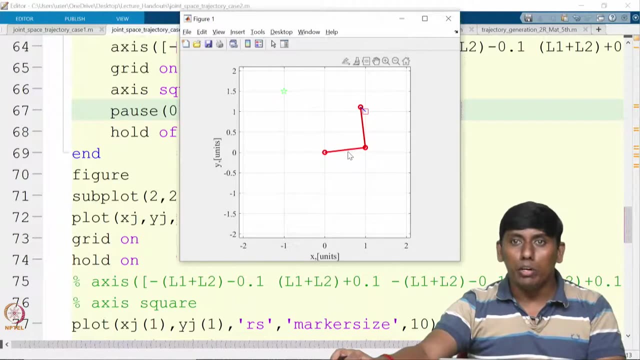 You can see like the first joint is rotated, the second joint is rotating right, So it is actually like little faster. So I will just make it the pass command probably 100 millisecond rather than the you can say 10 millisecond. So now you can see the first joint only rotate, the second joint is as, whatever this theta. 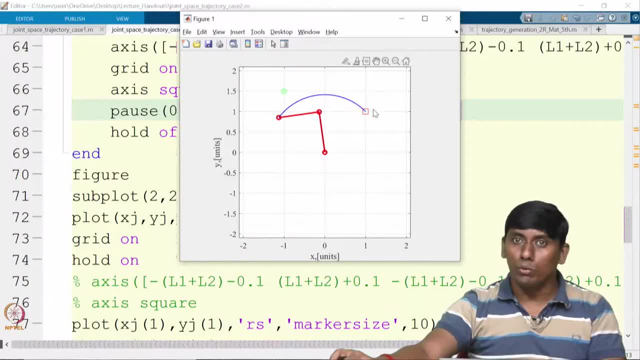 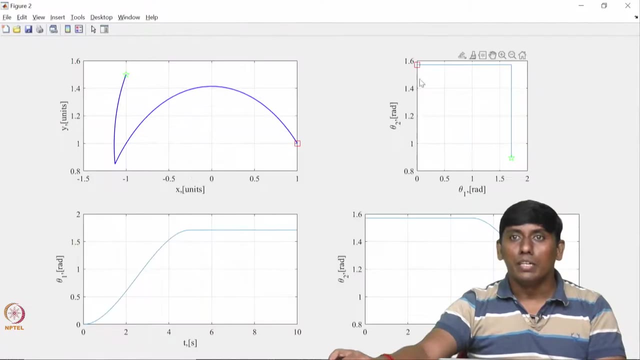 2: 0 is maintained. okay, the first joint rotated. Once it is reached that final, then it is the second joint rotated right. So while second joint rotate, you can see the first joint remains same right. So you can actually look at it So from here, so you can see like the first joint rotated. 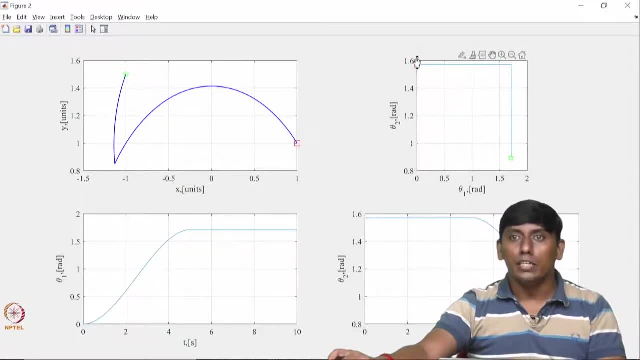 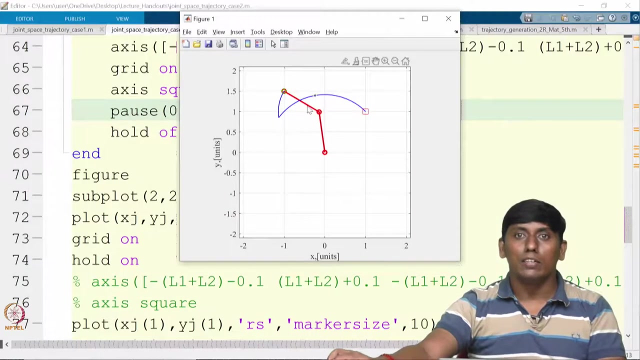 So that time the theta 1 vary, okay, From theta initial to final. So the second segment, so theta final, theta 1, final remains same, But the correspondingly theta 2 start from 0 to final. okay, So that is what the realization. 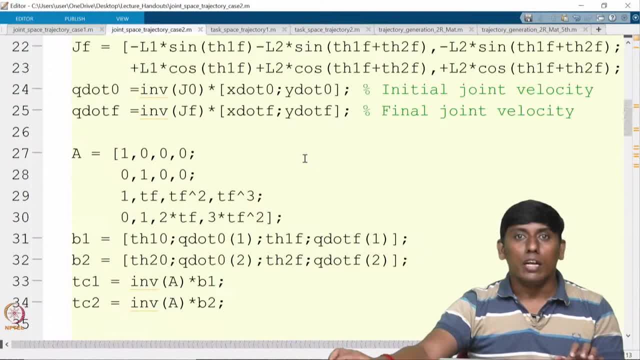 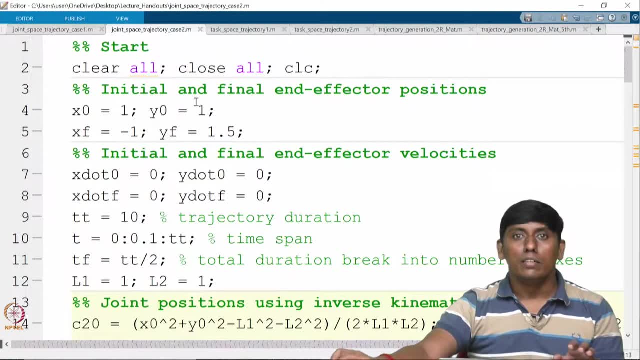 So now you can actually like want to more clear, So I will just give random theta 1f, So in the sense. so I just give it probably a different point, So I will just put it this much. Okay, So I will just show it. this is actually like vertical. 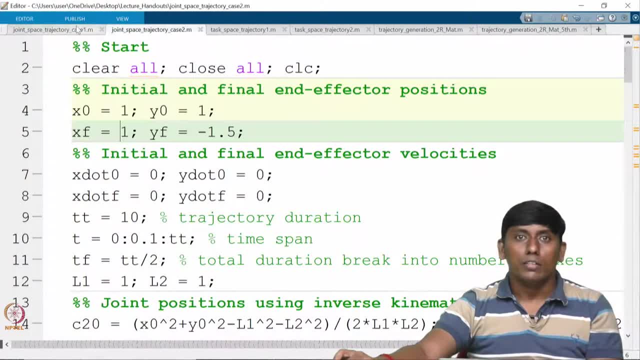 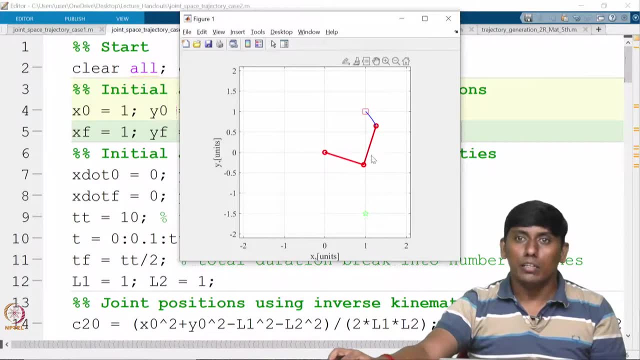 So then you can actually like see it. sorry, so you can actually like see it. while running it, you can see the first joint only rotating. the second joint remains same constant. So once it reached a particular location, you can see the second joint rotate. that time the first joint remains same right. 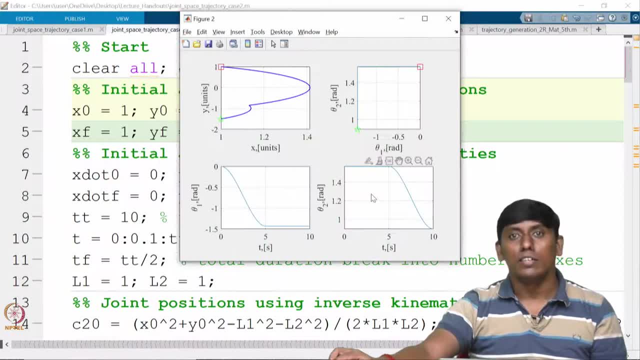 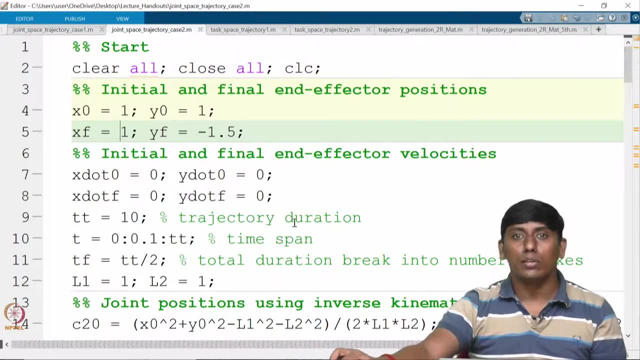 So it is very clearly see that the explicit prejudice, But this is not preferred at all, however. so most of the you can see kinematic solvers and all done with this way, individual joint would be move in series. So, especially if you go to Ross, we call robot operating system. 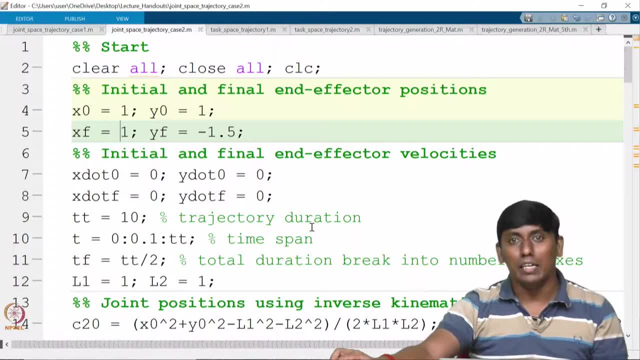 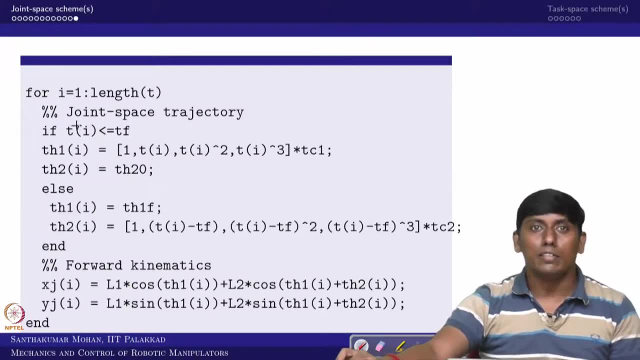 So I already told in the lecture these things all very clearly visible there. okay, So now going back to the slide, so we will see this. whatever we have seen is the joint space trajectory Can we see in a task space, even the task space we can actually like see in that case, 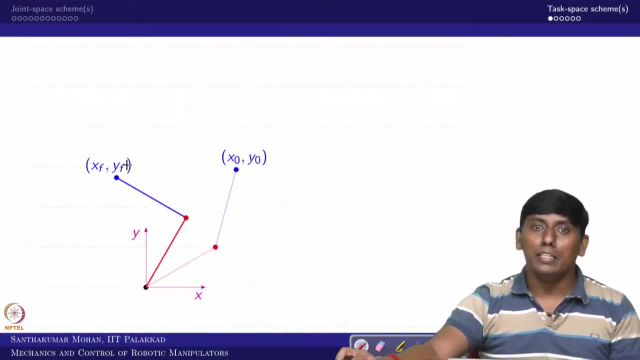 So x, initial and final, would be given. similarly, y, initial and final would be given. So this is the initial position and this is the final position. we want to follow this in the sense it is supposed to be followed at the straight line. So the straight line is not assured because x dot of 0 and x dot of f if it is non-zero. 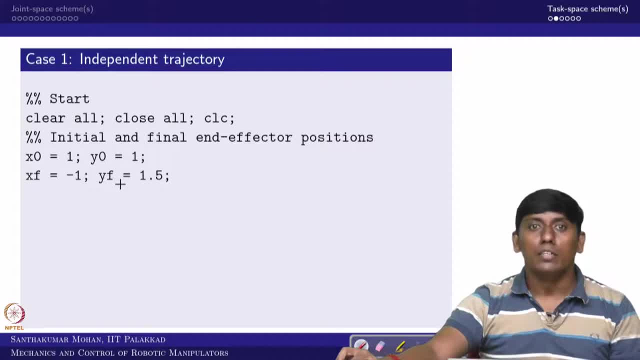 then it would not maintain. So we will see that how it comes. So in the sense here you can actually like see. So we are trying to do the first case, independent trajectory in the sense x trajectory and y trajectory. we are trying to do it in independent cubic polynomial, we are not doing it a synchronous. 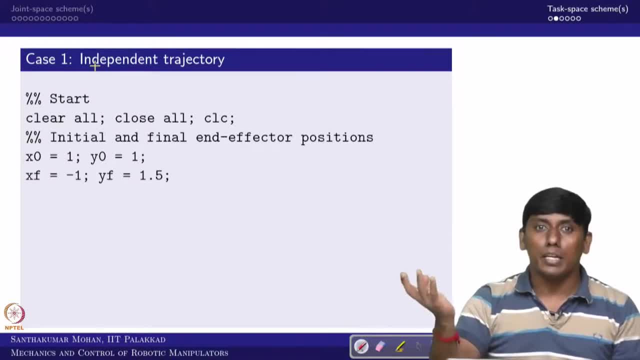 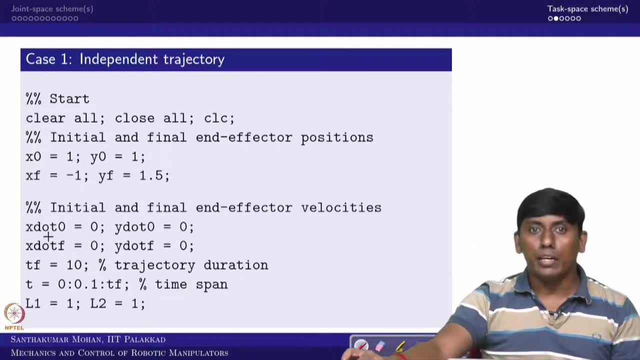 may, in the sense, once you do the x, based on the x, y can be generated. no, not like that, okay, So in that sense we are actually like trying to do this. so here you can see, initial and final velocity are given and we have taken the same time, which is phi, you can say. second, 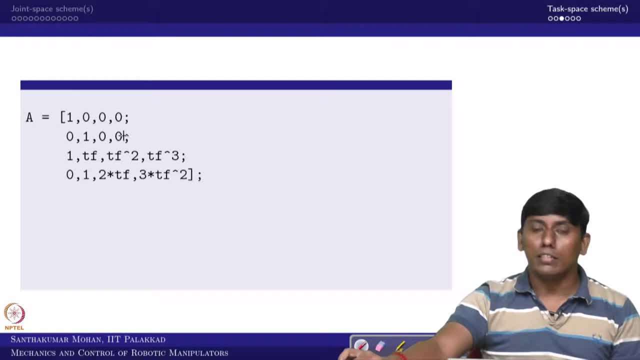 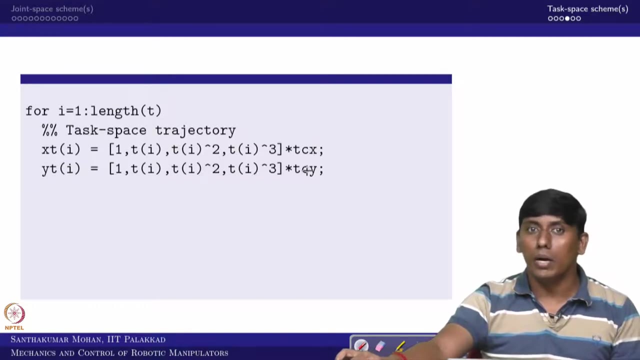 And l1 and l2 are same. So now we have taken the same a matrix, but bx and by are the two other vector, based on that, the coefficient, what we calculate, tcx and tcy. So now, in that case, so xt and yt, which is actually like written, as tcx and tcy. 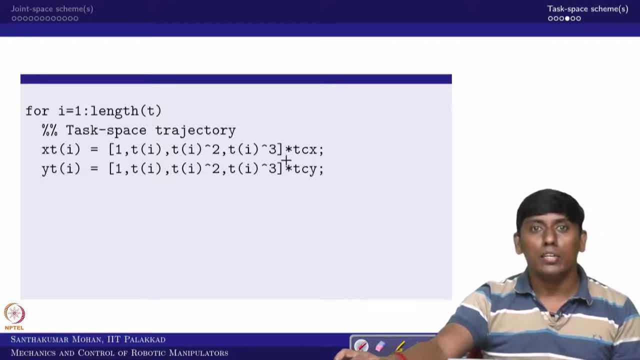 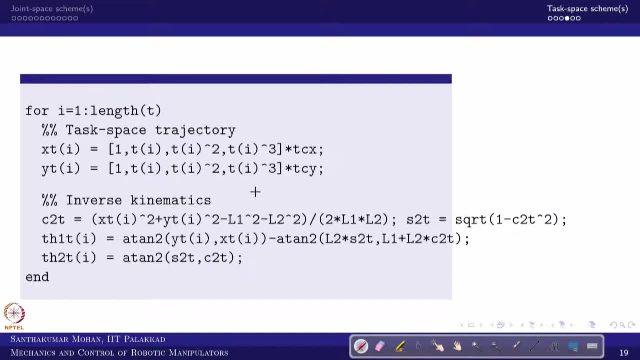 So, in the sense, the x trajectory and y trajectory independently derived. So, in order to check, in order to compare, so we have done the inverse kinematics, just to see how the theta profiles, Theta profile will go. so we have done the inverse kinematics. 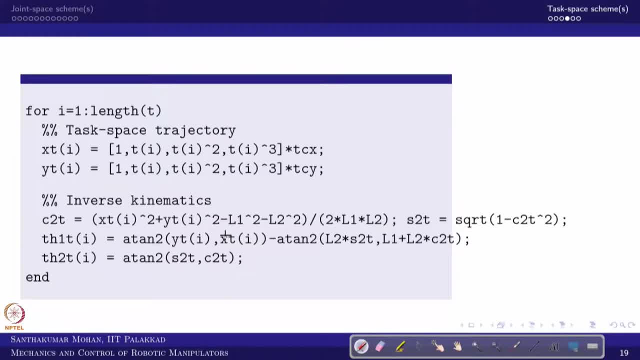 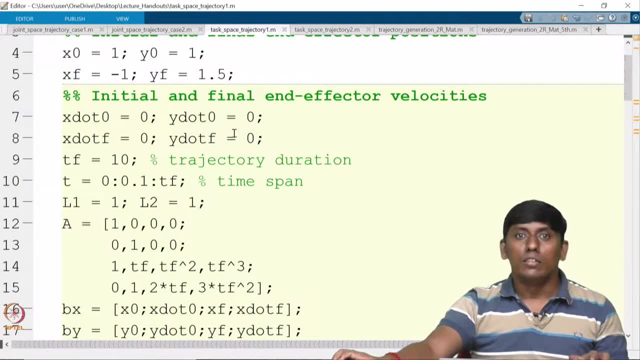 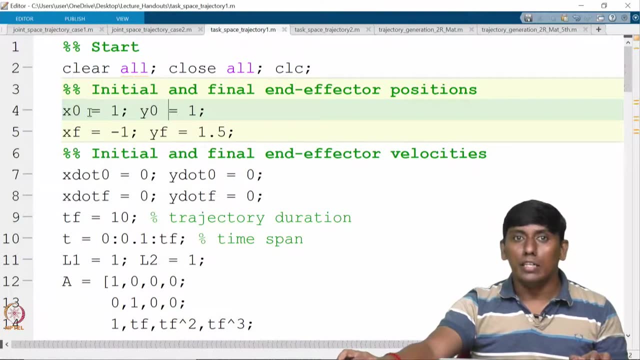 So now we have actually like use the same plotting command, So we will actually go to this, the task space trajectory one. So you can actually like see that. so these are the cases which we have shown in the MATLAB where initial and final. you can say initial and final, initial and final of y and initial. 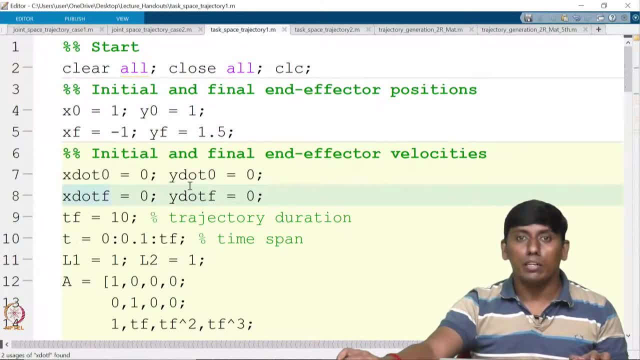 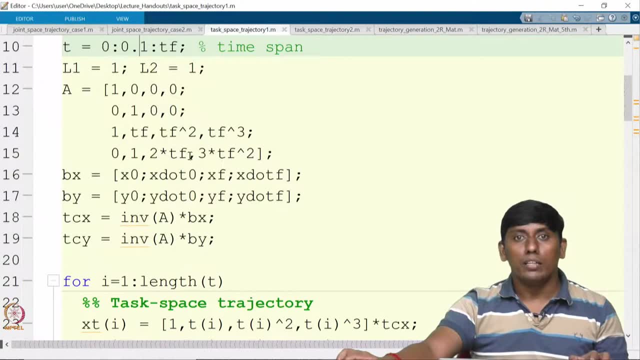 velocity of x and y and final velocity of x and y And The total duration is 10 second and you can say this: all we have tried And the a matrix, bx by are given and based on the tcx and tcy can be calculated and you. 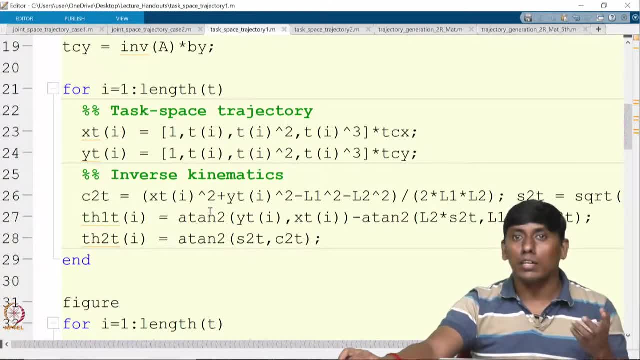 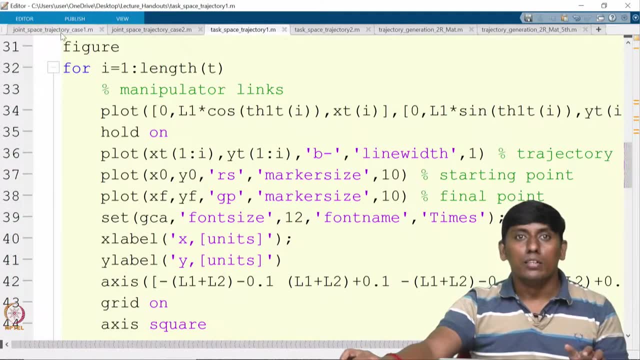 got the task space trajectory, Then the inverse kinematics, just for our reference. we calculate so that we can do the plotting option. okay, So the plotting option. we have used the same thing. So now, if I run. so what you have expected earlier it was a curved, now in this case it 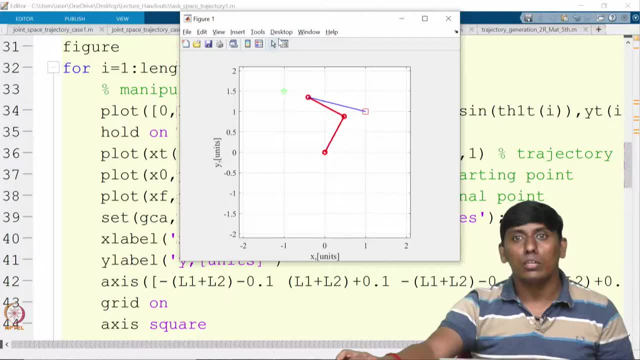 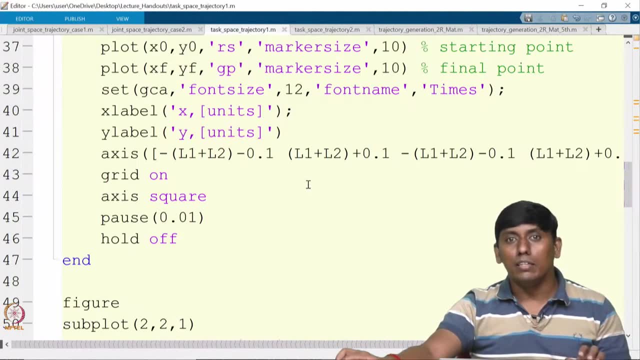 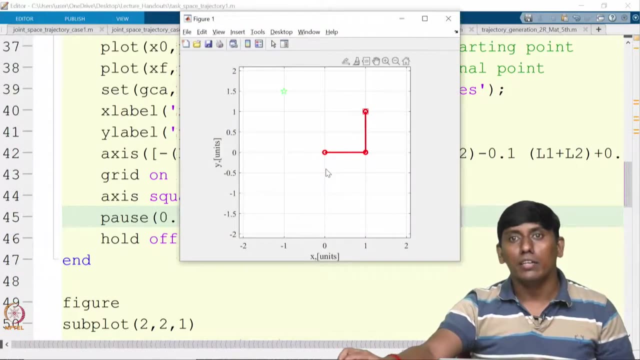 is a straight line which is followed, But the straight line is not assured if the initial and final velocity are non-zero. okay, So now you can actually like see it, So I will just make it. the time duration is actually like higher. So now, in that case, the delay time is actually like higher. 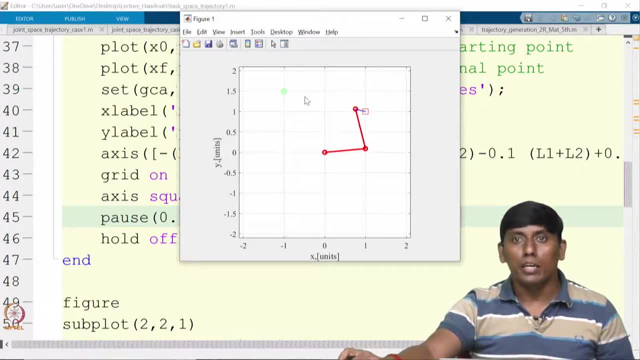 So you can see like it start from this point and it is supposed to go here. it is trying to follow a straight line because the initial and final velocities are zero. If the initial and final velocity are non-zero, what will happen? you can actually like see. 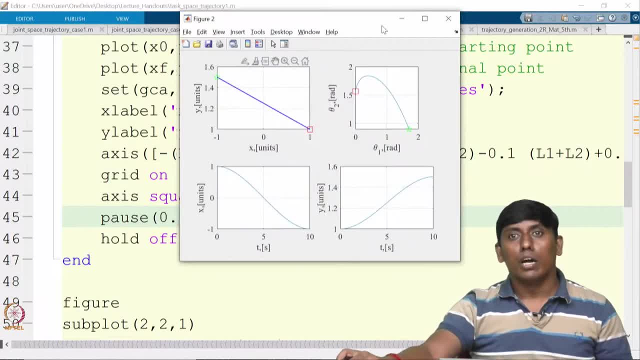 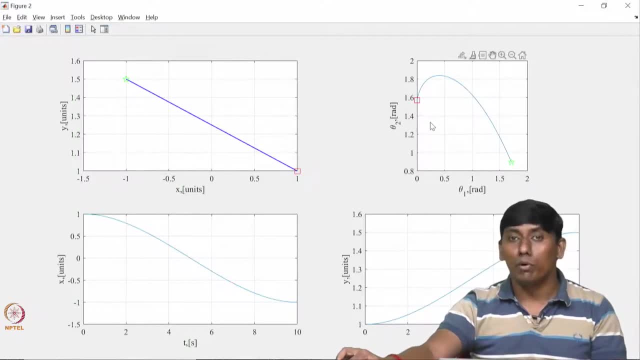 it by changing that. okay, So now in that case you can see there is a joint space. you can see like it is not following as a straight line. earlier case: it was followed as straight line. Earlier case: the task space trajectory is followed as a curve, but in this case is a. 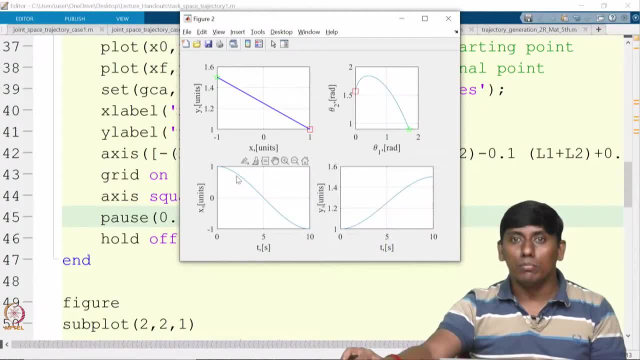 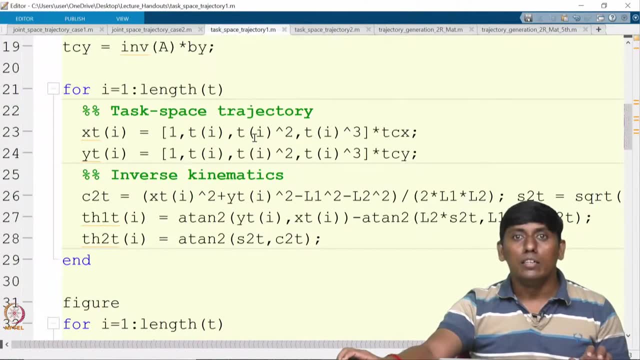 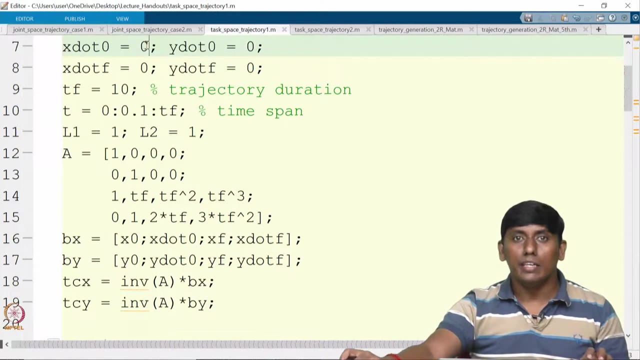 straight line, right. So the same way, x trajectory is smooth, y trajectory is again smooth, these all we can realize it. So just to show that, how the non-zero initial velocity will involve, So I am just saying that only so the non-zero x is there, which is actually like 0.5 meter. 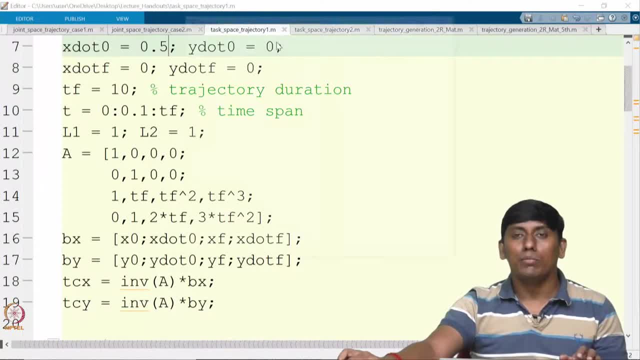 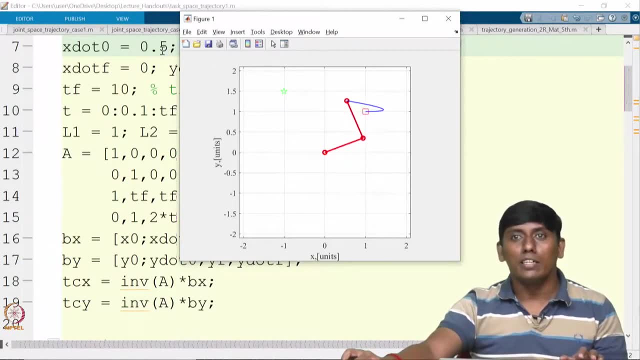 per second. So you can see that it would not be straight line. it would be giving a small curve because it is actually like already having some non-zero initial velocity. you can actually like see that it is trying to follow however it is going to. at rest, it would not get any residue. 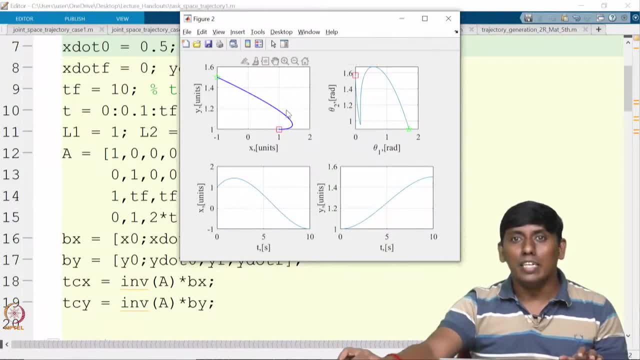 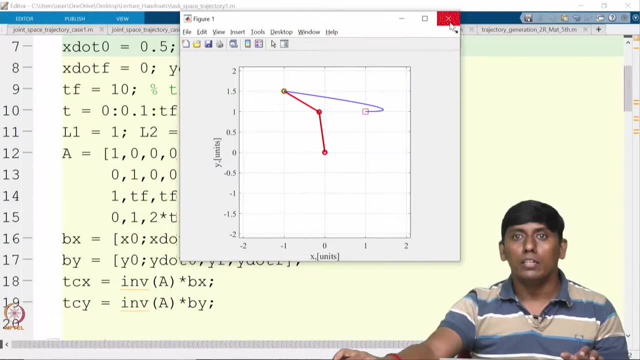 there, but here it is starting from non-zero. you can see that the profile is actually like invariantly modified. okay, So that is what you can actually like. look at it. So even if I give something like the final velocity of this, I am just giving randomly. 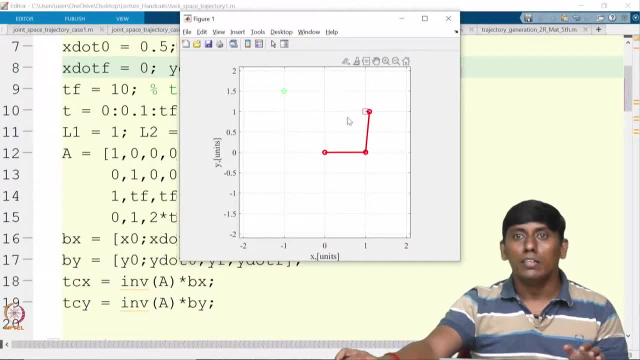 So the y final velocity is 0.5 meters per second. So you can see like it is actually like for the x axis. it is there, So that is why it is trying to go and now you can see it is modified because the y final 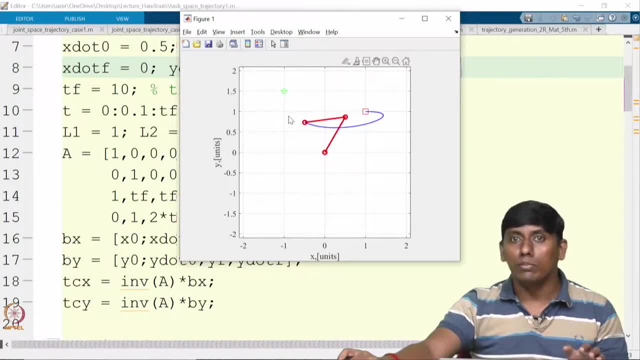 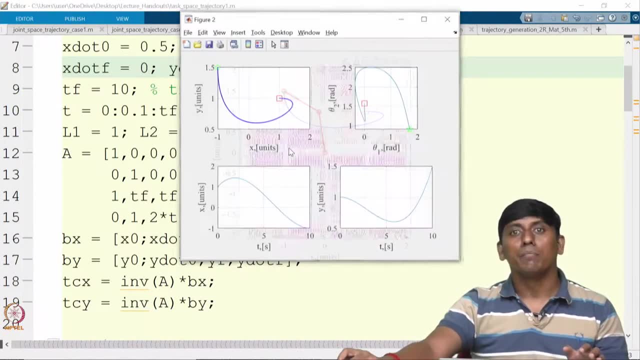 velocity is supposed to be somewhere 0.5 meter per second, So in the sense, vertically up, Okay, So that is why it is start from horizontal and end with vertical. that is what it is showing, okay. So now you are actually like- I hope you are actually like getting the clarity. 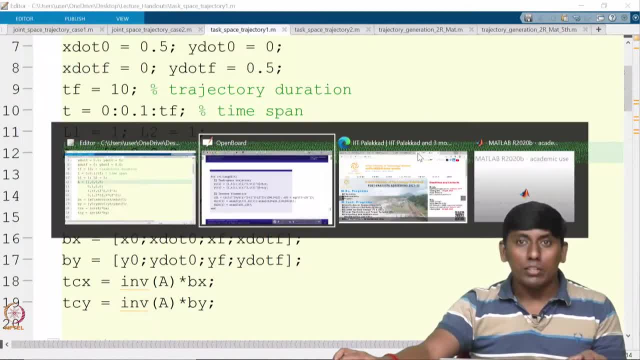 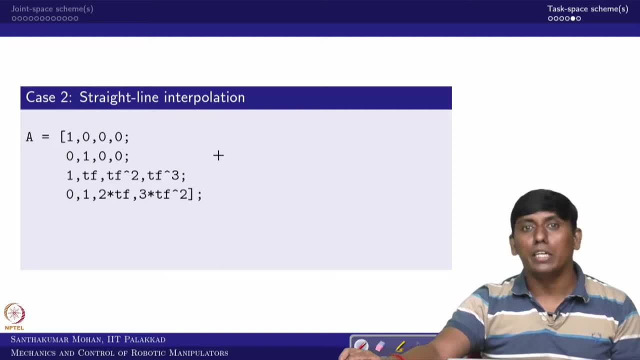 Now we will actually like move to the second case. What is the second case? So where the straight line interpolation, so the straight line interpolation, only one modification we can expect. So what modification? so instead of this? so we would be having derived from the x. 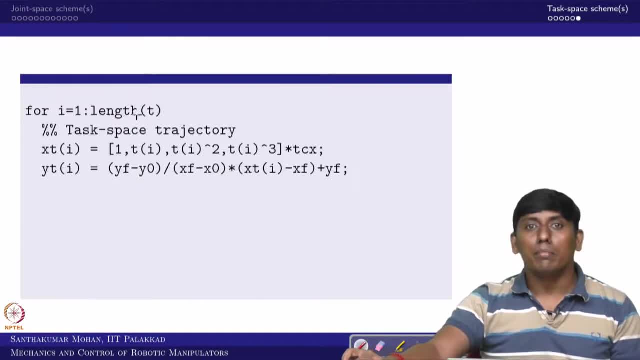 So you can actually like make only x So then we can actually like make it y So based on x So, which is what we have done in a straight line interpolation, if you recall. So, if once you know this, so you can see like the x of t is derived based on the x of t. 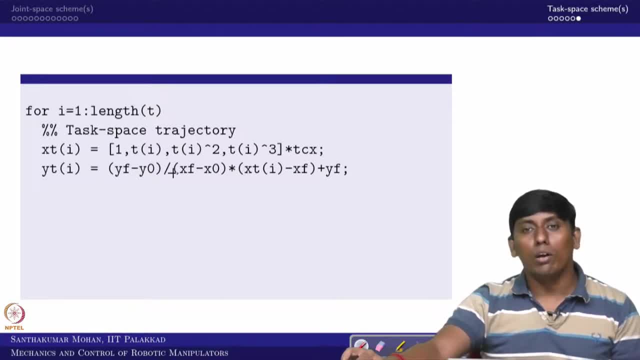 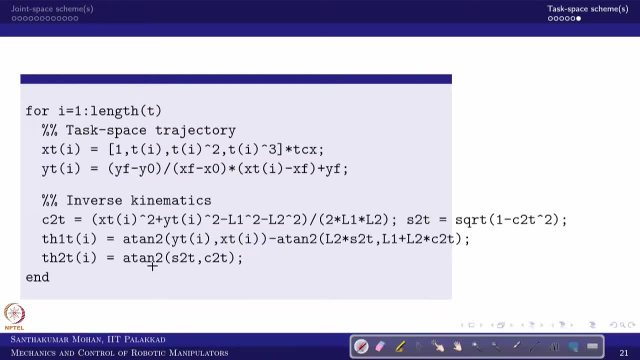 the y of t is come. So in the sense, y, dot and all will not come explicitly here. Okay, So now, in that sense, this is the inverse kinematics, the standard, And we have actually like The same plotting function. we will be using it. 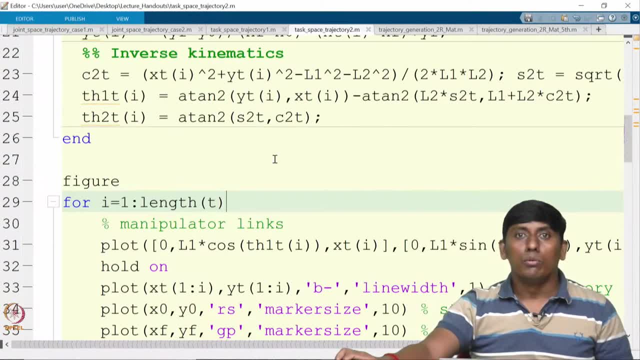 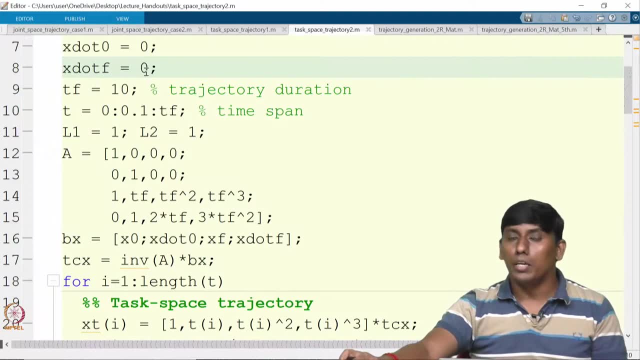 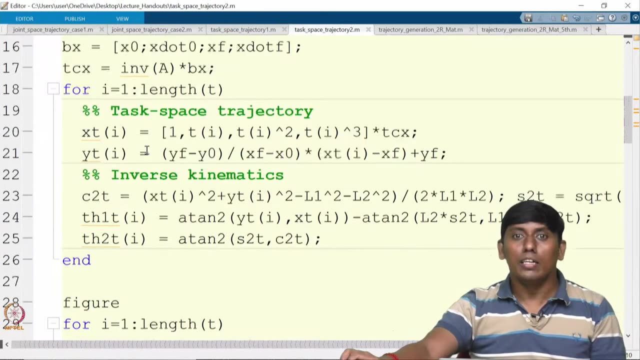 So the task space, trajectory 2, you can look at it. So this is what the given condition, So the same condition we have taken, and x dot and y dot only, like x dot initial and final, only we are taking for the trajectory generation. So then we are actually like deriving the y of t or y. 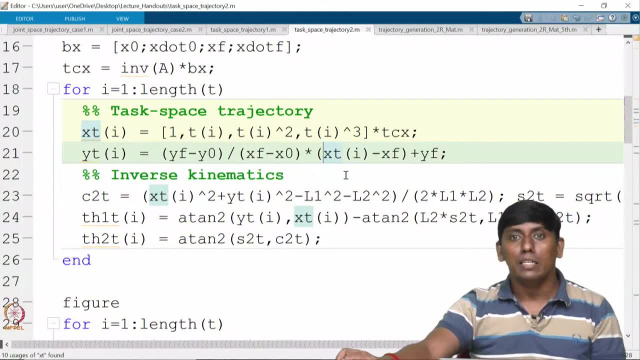 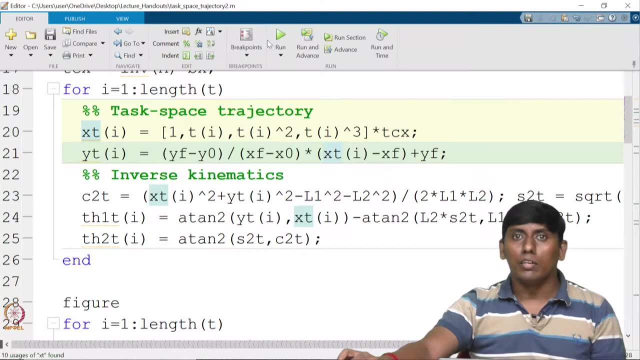 So based on x. so that is what you can see explicitly. So then we are actually like moving to the Same thing. So now you can actually like look at the profile, which is actually like going to be very smooth because the y would be given. 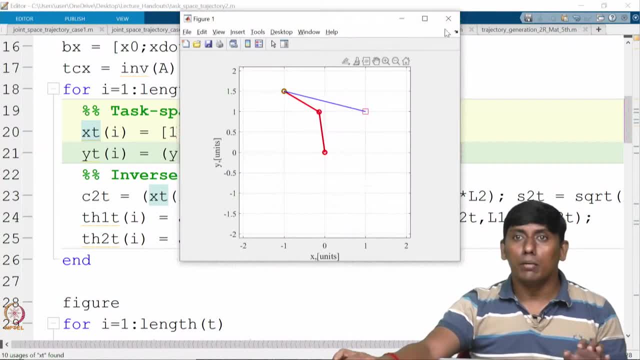 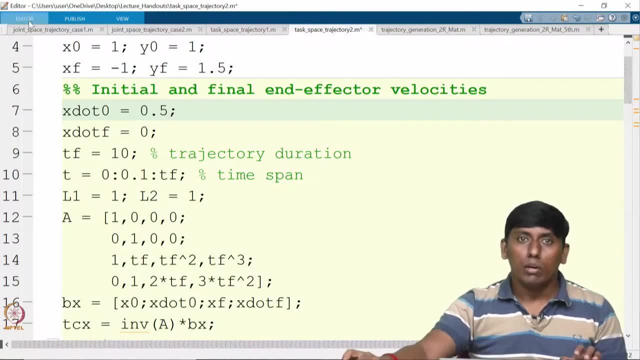 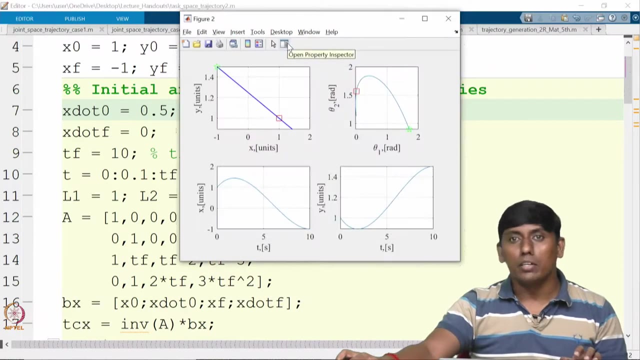 So now you can actually like feel it. So now, even if I give some non-zero initial velocities- So for example, I am just taking it, this is 0.5.. So now the profile would be, you can say: goes like that. however, you can see, the y is not. 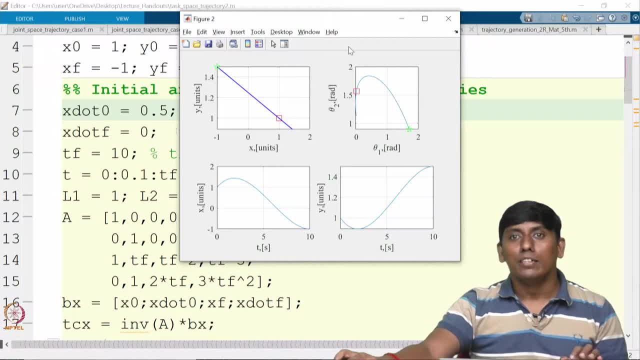 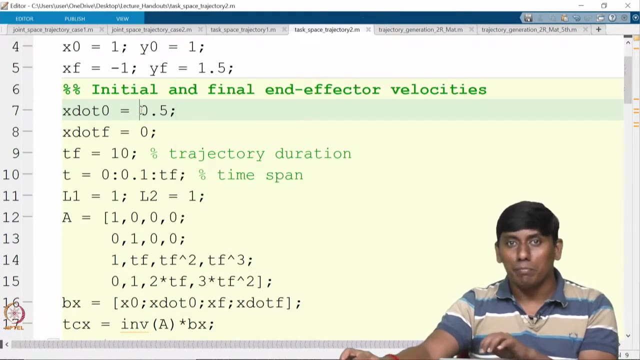 coming right. So that is what you can actually like feel it. So it is actually like going across the line and goes because you do not have any. you can see case, because we assume that this is actually like followed on the same line. For example, if I take minus 5, okay, 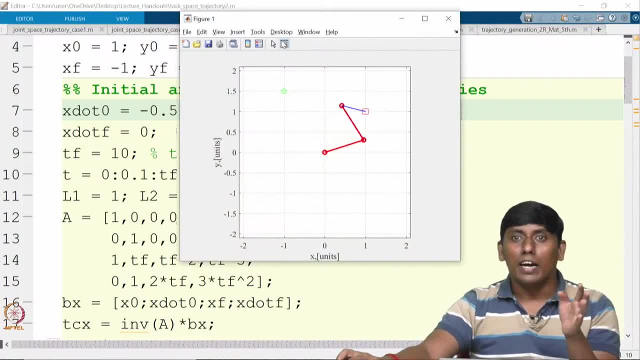 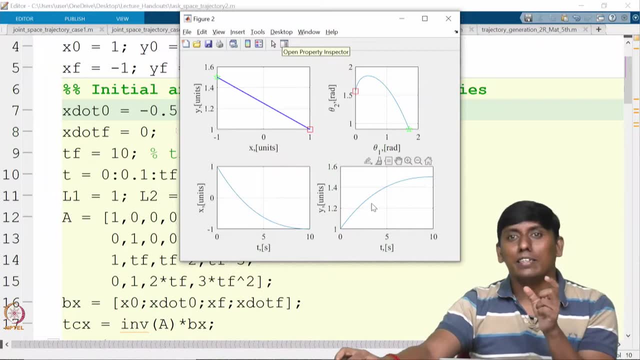 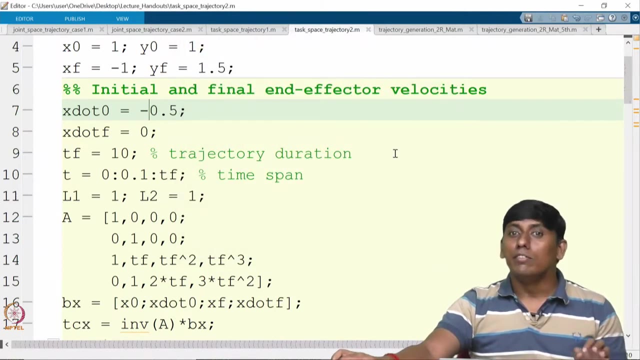 So you can actually like feel it that would be come on the same line and actually like go. So there is no change in your velocity, only thing this profile has interchanged. okay, that is what you would have actually like felt. So this is what the you can state line interpolation, even the state line interpolations you want.